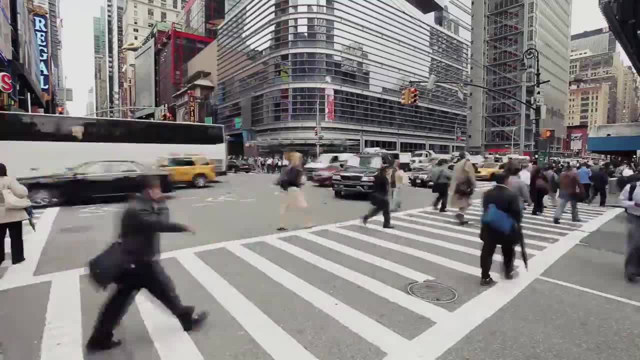 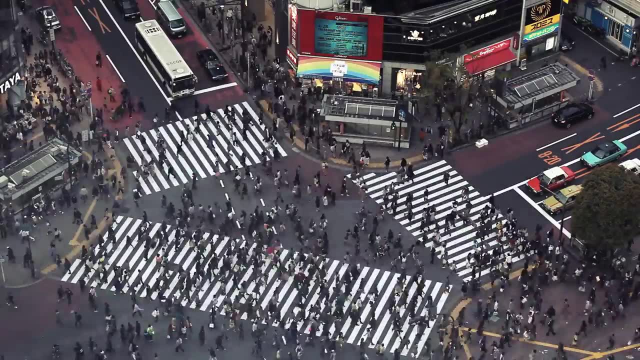 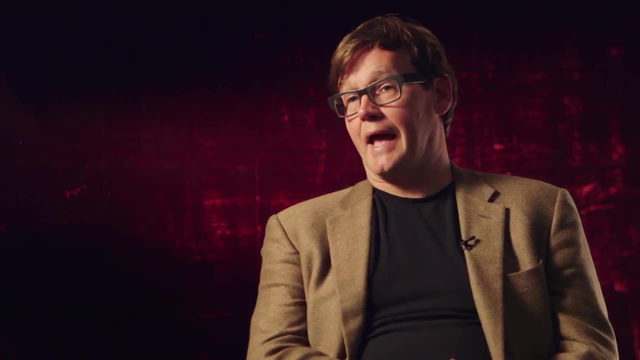 Without additional mitigation efforts, global mean temperature could increase by about 4 degrees Celsius within this century. The world economy right now is causing massive quantities of greenhouse gas emissions and they're going to keep on rising. To stop climate change, we need to cut them in half globally by mid-century and further after that. 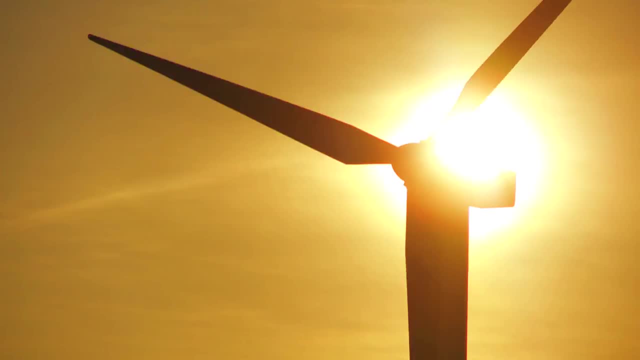 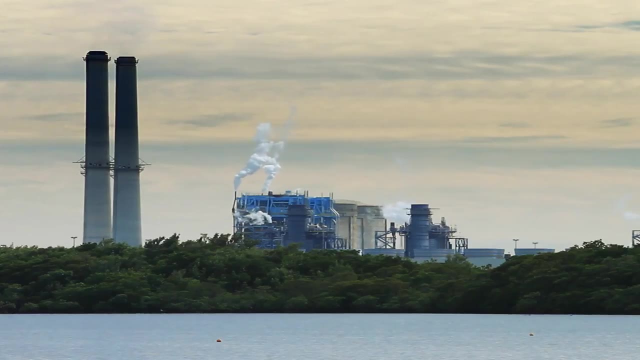 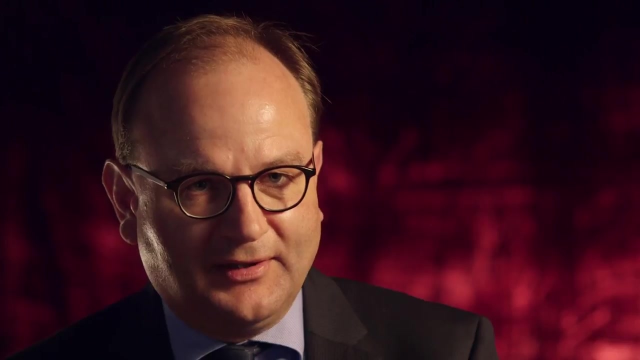 And that's going to involve complete transformation in the energy system, especially in electric power: New kinds of power plants, bigger, longer, more complicated electric power plants. The report shows very clearly we need a fundamental departure from the business as usual scenario. 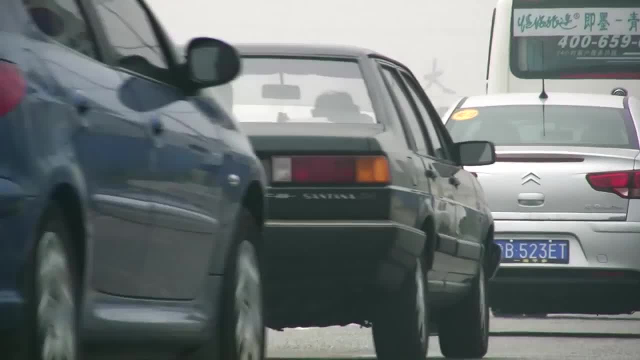 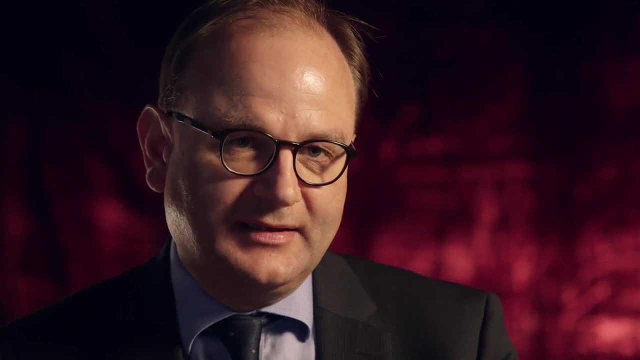 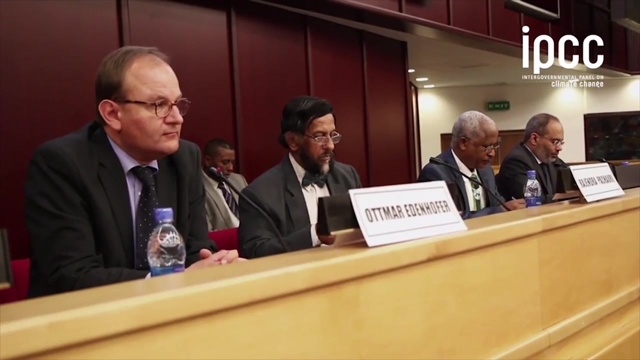 The policy makers. they refer in their policy to the two degree target as a kind of a focal point, And we provided the information and the underlying requirements to achieve this two degree target. The authors have analyzed a broad range of scenarios from the scientific literature leading to different levels of global warming. 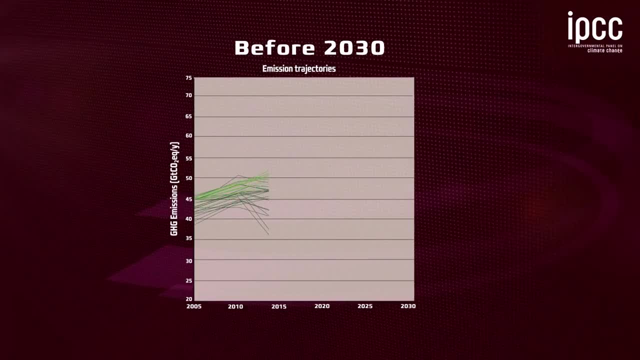 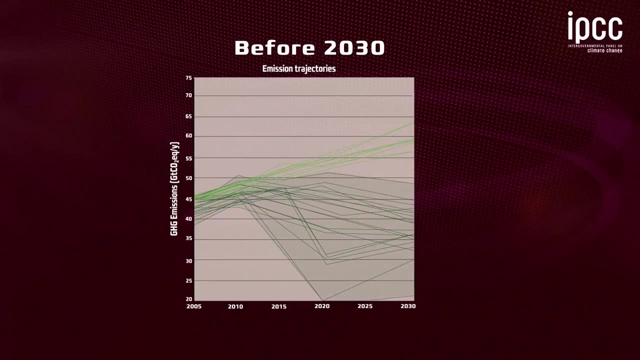 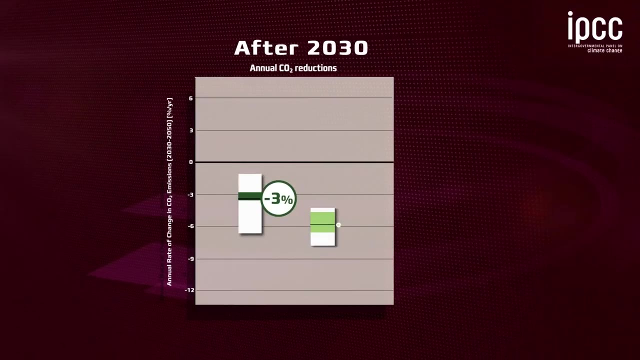 Many of these scenarios have emission trajectories that limit future global warming to about 2 degrees Celsius. The defining difference is the beginning of emission reduction before or after 2030.. If mitigation is postponed until after 2030, the necessary emission reduction rates will be about twice as high as in scenarios with immediate action. 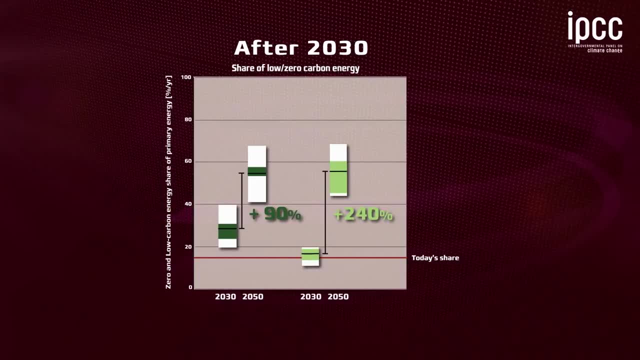 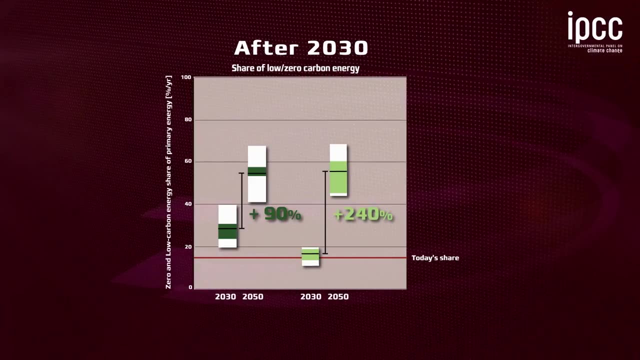 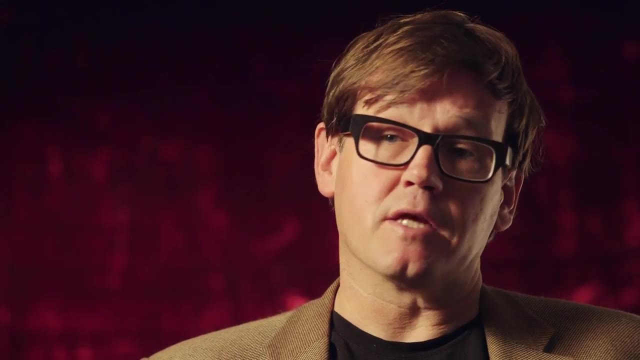 Reducing emissions means producing more low carbon energy. Doing less before 2030 means having to do much more in the following two decades. The analyst community is now much more aware of the complexities of designing and implementing policies And unfortunately that's also made us much more pessimistic about the speed and ease and cost. 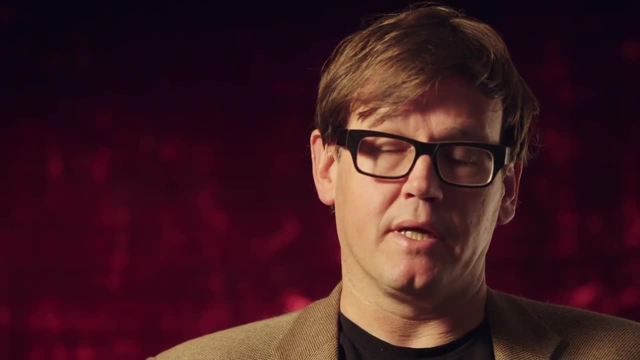 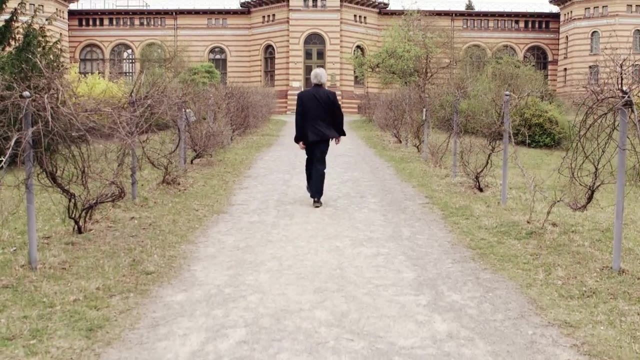 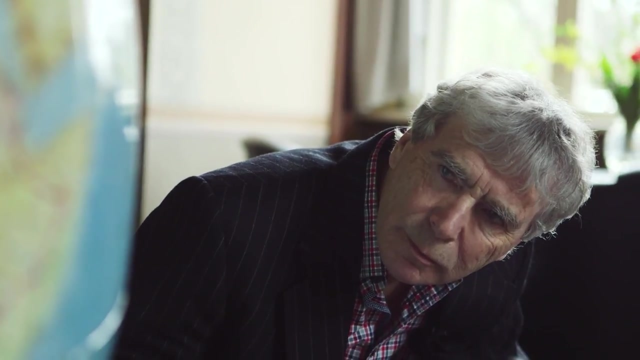 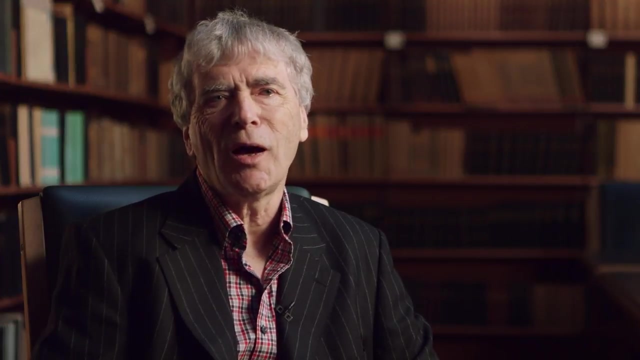 with which countries can adopt aggressive policies that will be needed. You can think of the atmosphere as a common resource. It's not owned by anybody. People around the world share it. They use it for various purposes, and I'm sorry to say that one is they use it for dumping their waste greenhouse gases. It costs each individual nothing To dump her gases and it costs nations very little to dump their own gases into the atmosphere. But the harm done by that is borne by people all over the world. That means the atmosphere gets overused as a dump for greenhouse gas. 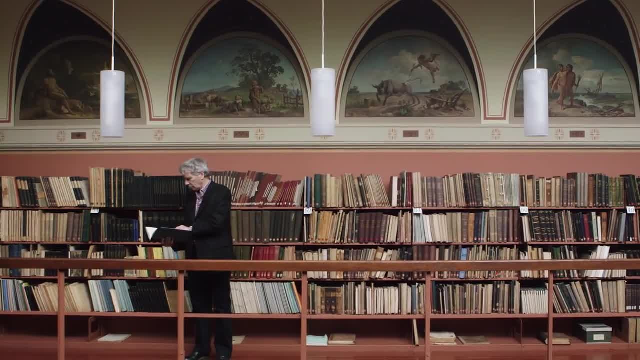 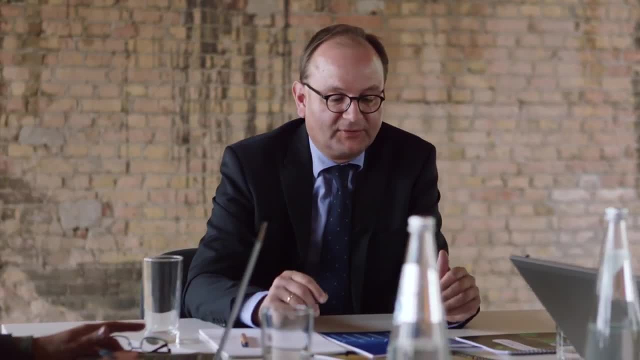 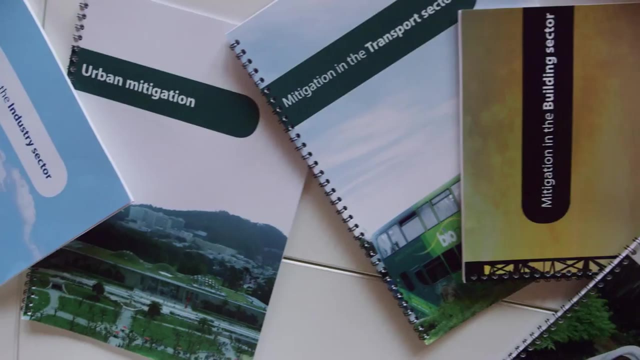 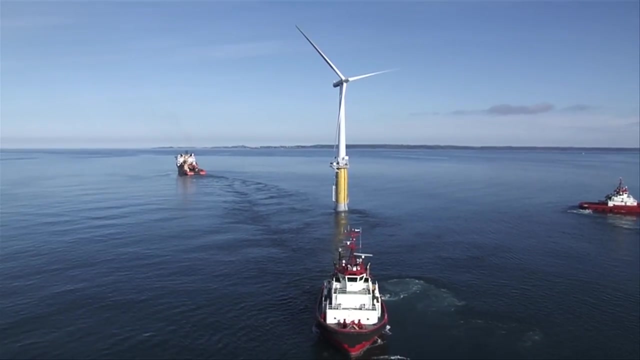 And that is the tragedy of the common. We have to find a way of reducing that. We need a broad portfolio of technologies, ranging from renewables, carbon capture and storage, nuclear power, energy efficiency improvements and a transformation of almost all the sectors. In the long run, GHG emissions from energy supply need to go down towards zero. 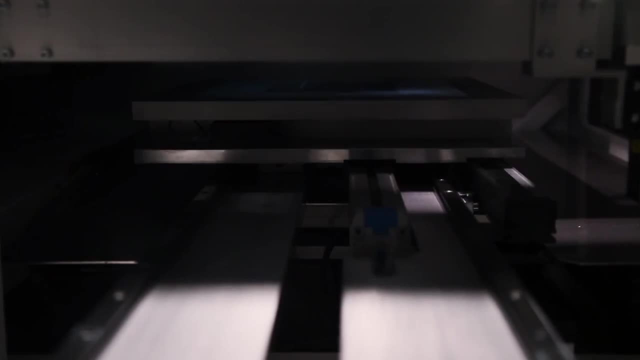 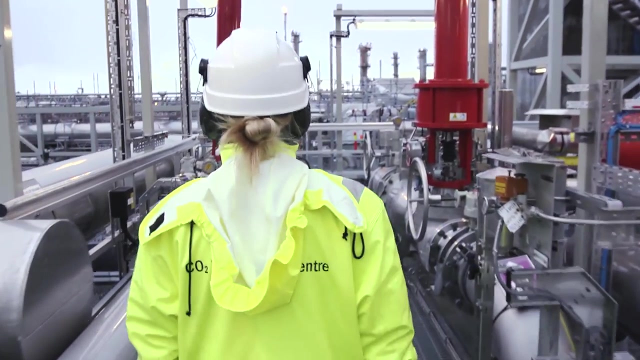 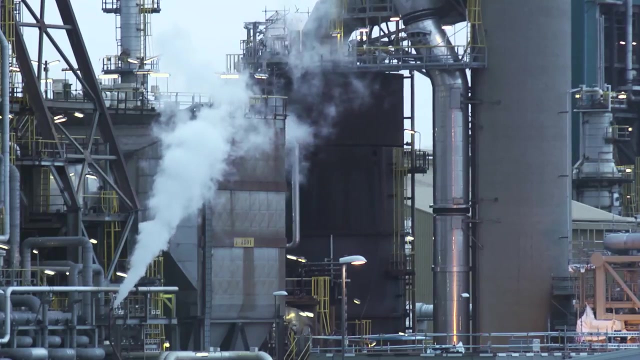 Advances in performance and cost have made renewable energy a fast-growing category in energy supply. Carbon dioxide capture and storage could be used to reduce emissions of fossil fuel power plants. The technology could be important for ambitious mitigation targets, but it's not yet been demonstrated at large scale. 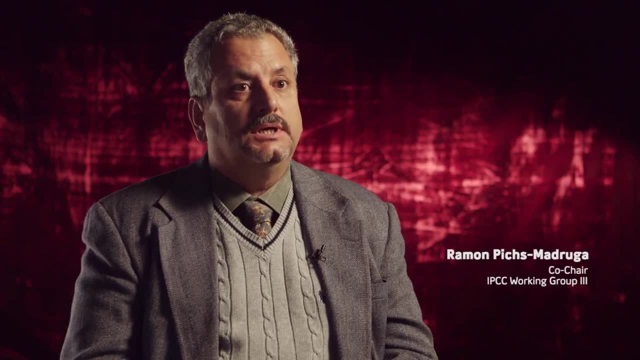 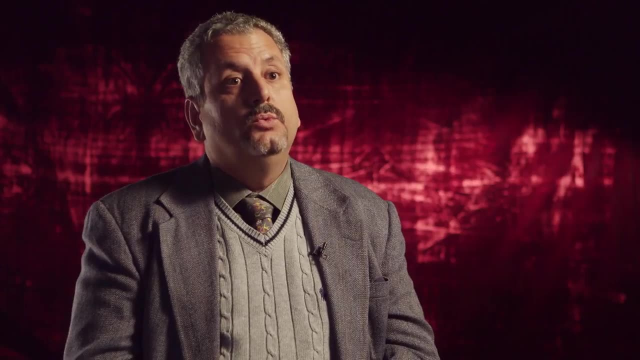 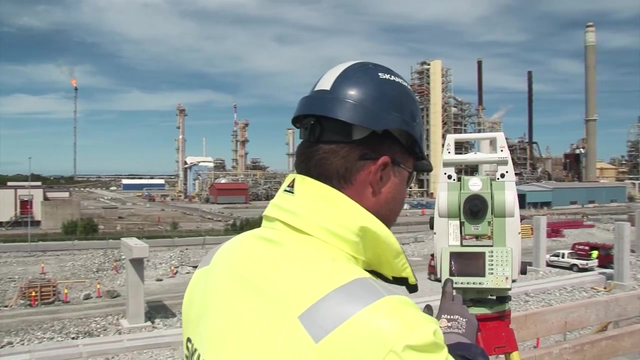 For implementing carbon capture and storage at a larger scale. it is important to take into account the need to compensate the operational investment cost with, for instance, higher prices of carbon markets, and also to take into account the need to consider the regulation needed to deal with the technological risk associated to this technology. 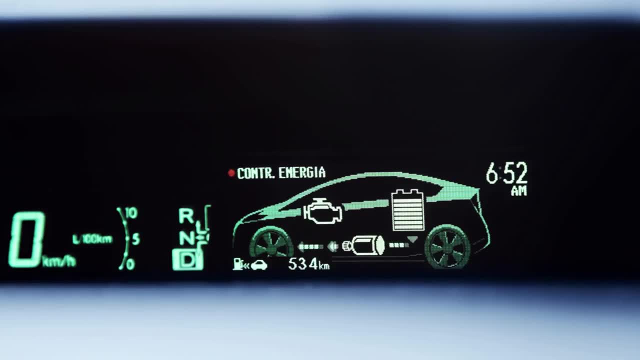 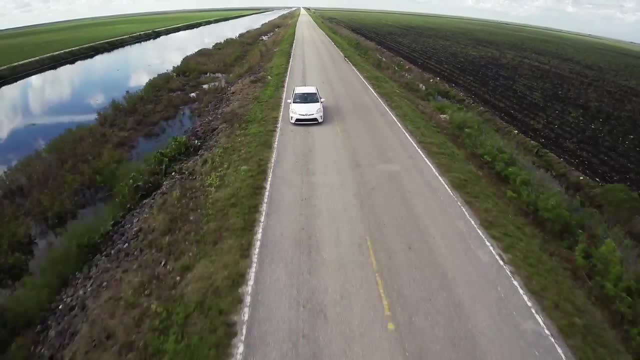 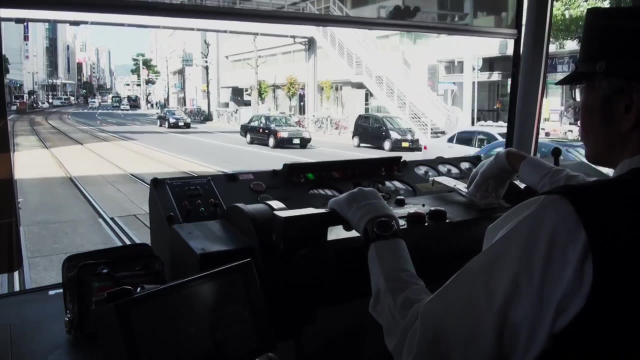 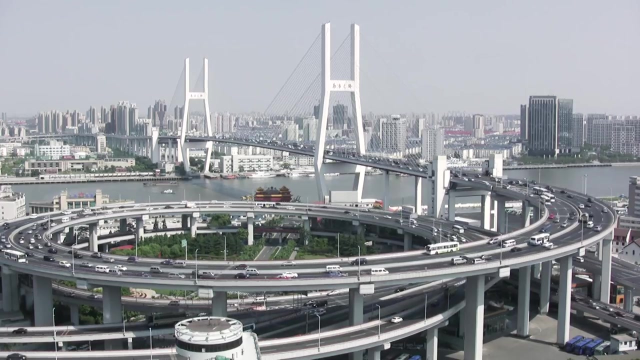 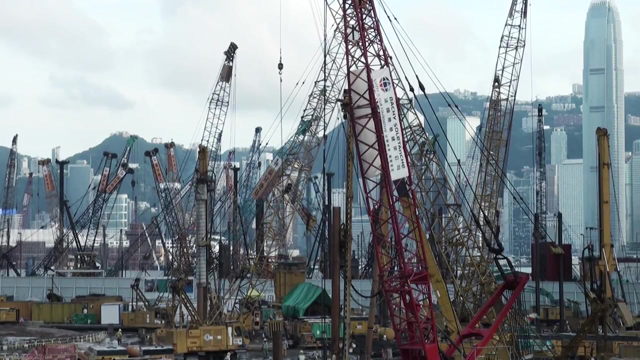 In the transport sector. the development of engines with low or no emissions and the use of new energy sources for transport are already happening. Technical and behavioural mitigation measures, in combination with investments in new infrastructure and urban redevelopment, could reduce energy demand substantially. Well, there are significant opportunities for urban mitigation. 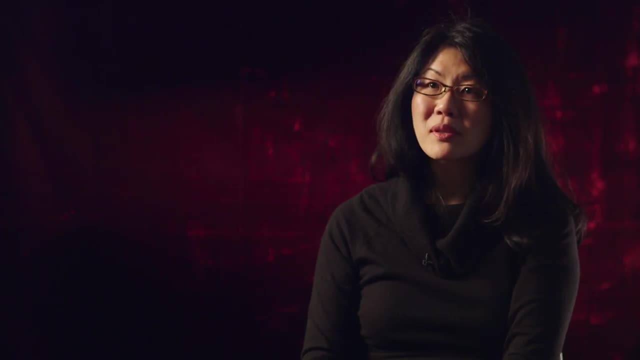 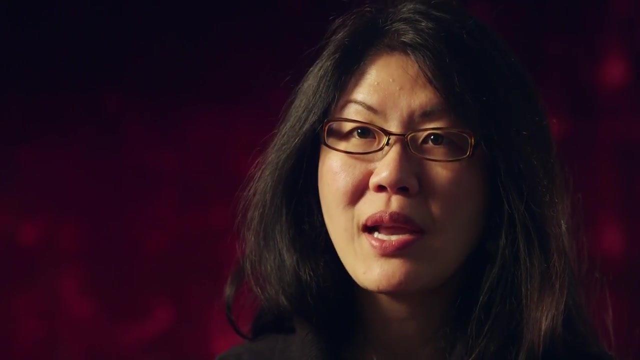 largely because most of the cities of tomorrow have yet to be built, And so we really are at this pivotal moment where, over the next 20 to 30 years, there are many countries, especially in Asia and Africa, that will be developing and constructing their roads and infrastructure. 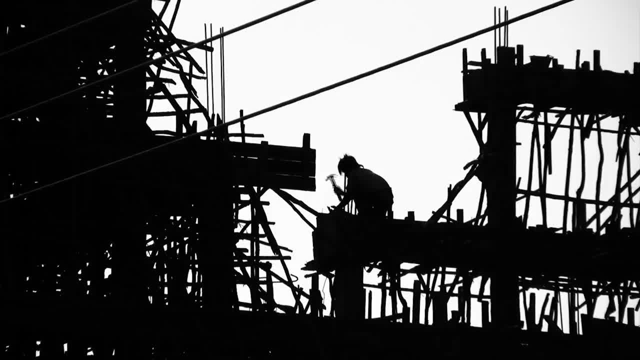 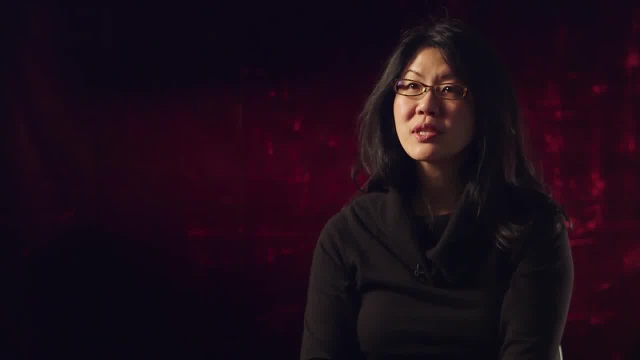 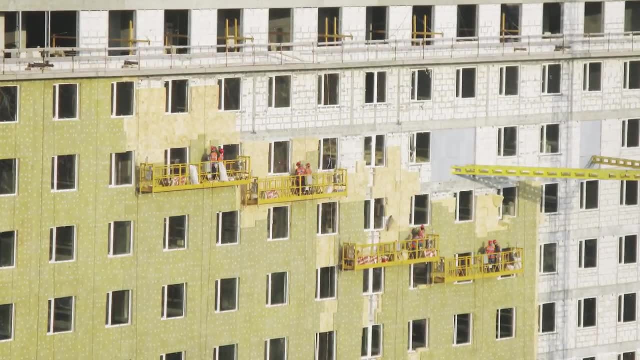 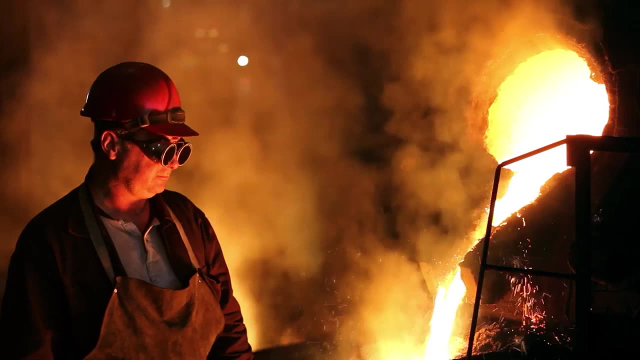 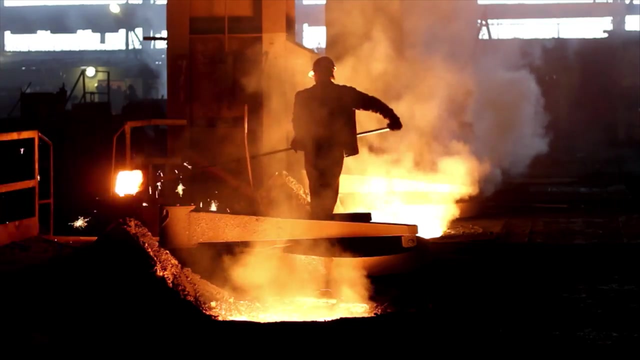 Some of the main mitigation options in the building sector are really associated with the significant improvements in building performance, increases in energy efficiency and really a reduction in building costs, such that it makes it much more financially feasible to retrofit inefficient buildings. In 2010, about a fifth of the total global emissions came from industry. 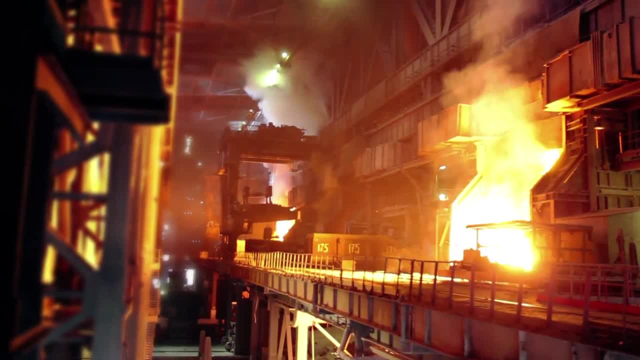 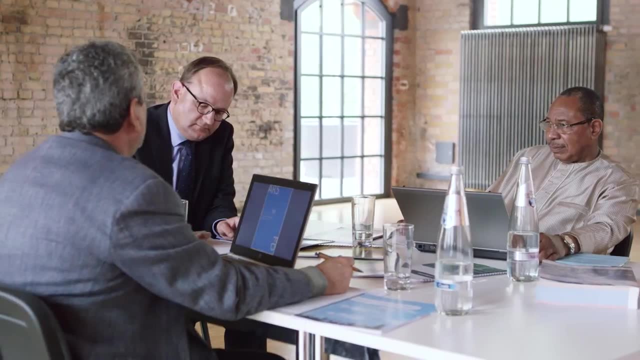 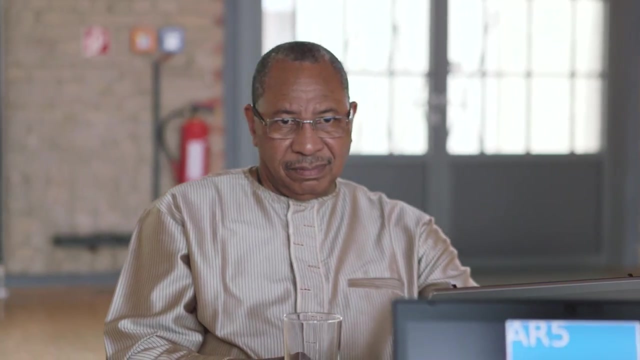 To reduce total emissions, energy, materials and products would have to be used more efficiently, And there is one aspect which is particularly relevant in the case of the industrial sector, which is the role of innovation. It is important, firstly, to remove as much as possible. 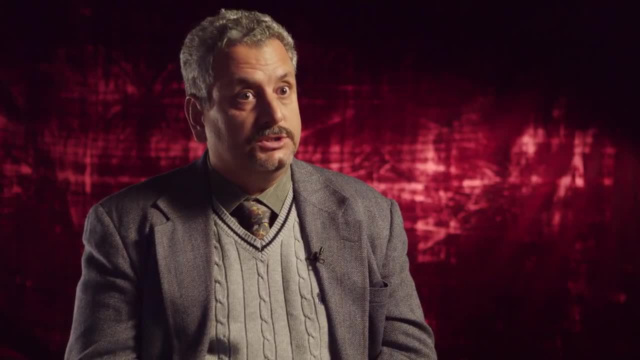 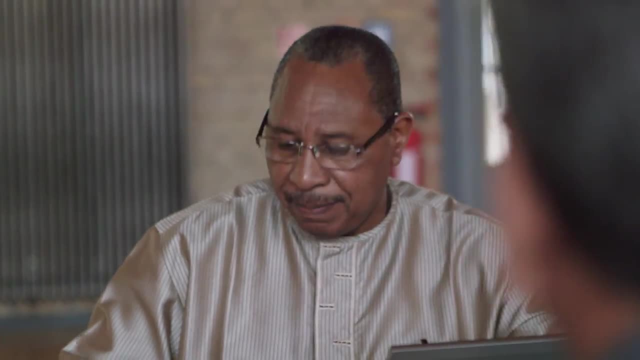 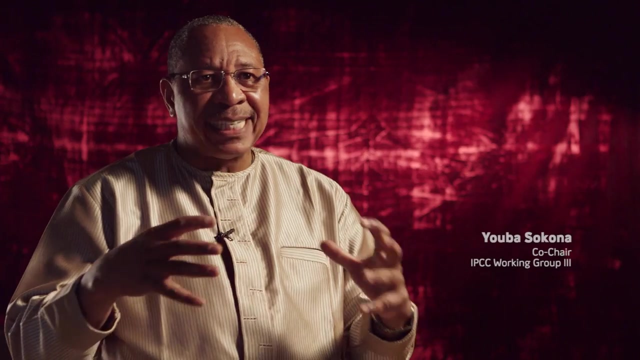 decision barriers, for instance, the initial investment cost, and also informational gaps. To achieve ambitious mitigation targets, policies need to be implemented across all sectors of the economy. There is interlinkages between different sectors. Cross-sectoral mitigation is much more economically efficient than sector-by-sector specific. 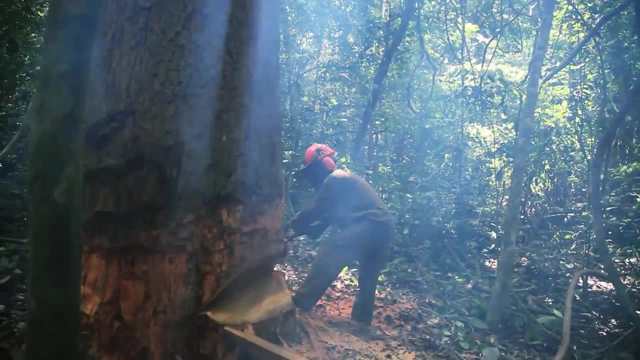 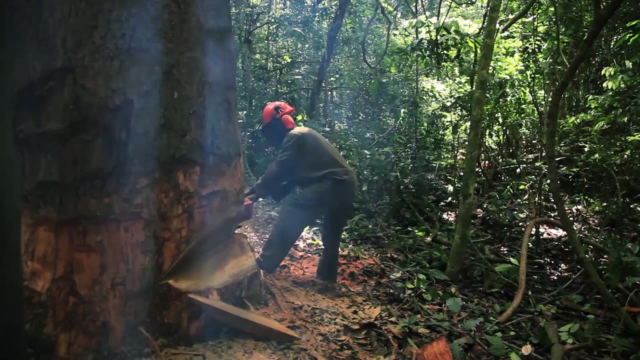 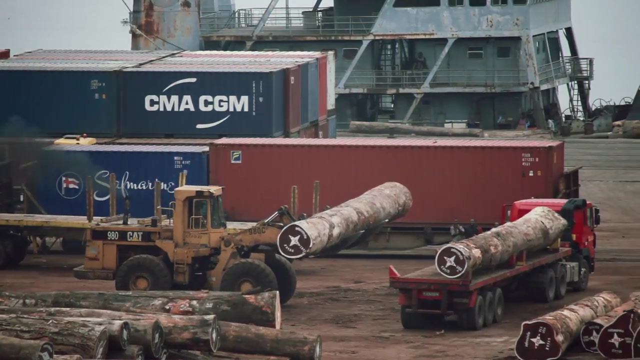 About a quarter of GHG emissions come from agriculture, agriculture and forestry. Deforestation is a large source, but the related emissions have been declining in recent years. Land use is a unique sector that offers many different options to reduce emissions and also ways to draw carbon dioxide from the atmosphere. There are two sets of major mitigation routes. One of them is afforestation, So you plant wood, for instance trees, in the tree groves. to a certain point it picks up a lot of carbon. That's one option, But the other measure would be to take that tree. 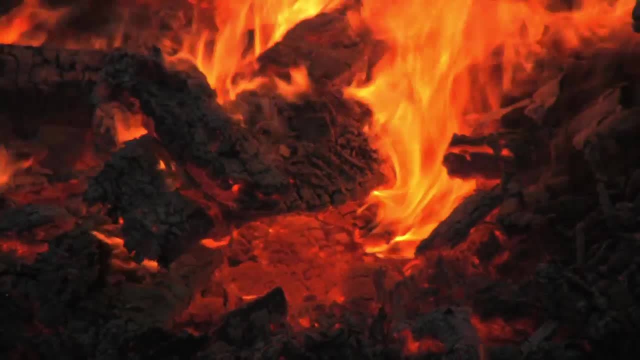 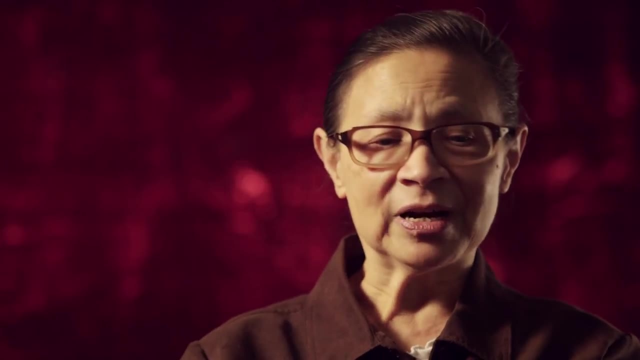 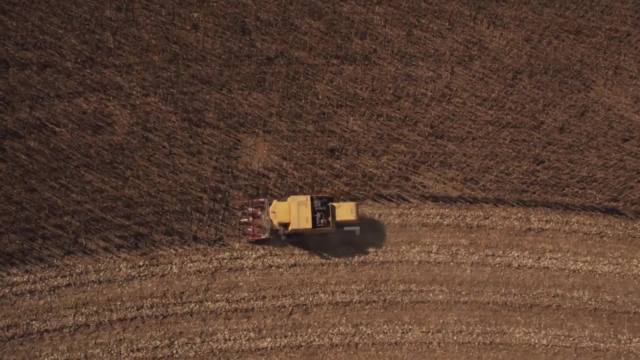 and then convert it to energy, but capture all that carbon dioxide and sink it into a geologic storage. So that's called BEX: Bioenergy and Carbon Capture and Storage. that would provide negative emissions As emission reductions are postponed. the use of bioenergy in combination with carbon capture and storage. 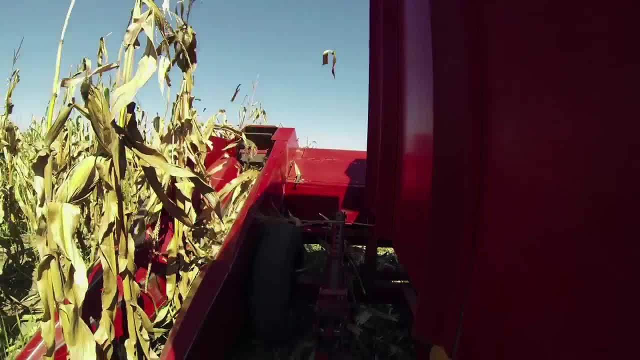 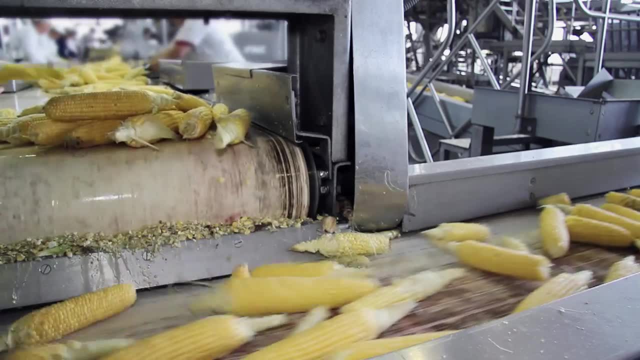 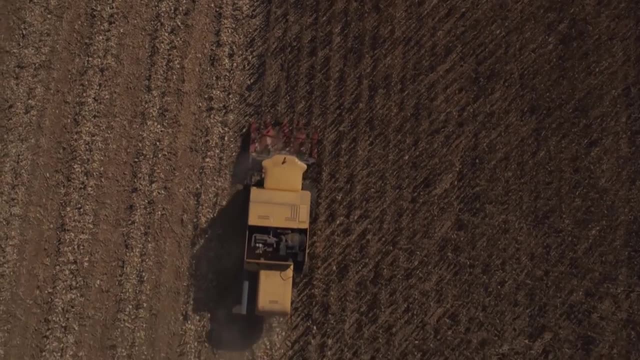 is becoming an increasingly important mitigation option, But upscaling bioenergy production comes with risks for food security, water resources, biodiversity and livelihoods. The sooner emissions start declining, the less will depend on risky negative emission technologies in the future. There can be significant risks associated with large-scale mitigation measures. 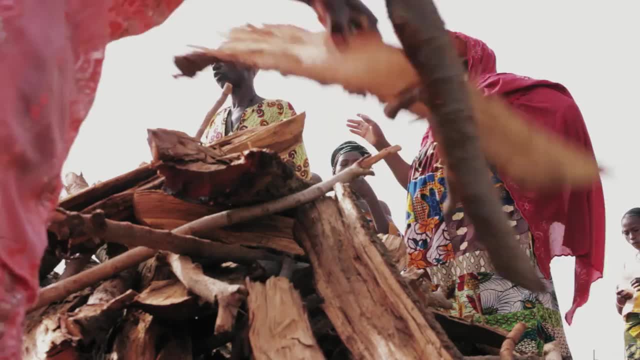 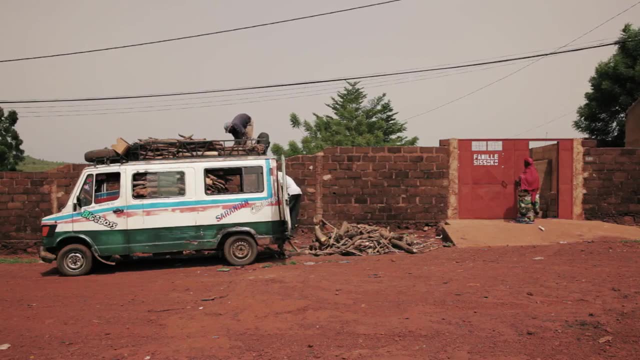 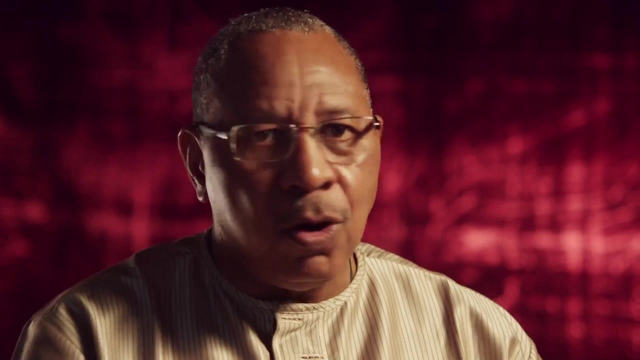 But on the other side, there can be benefits beyond curbing negative climate change impacts. Let me take the case of Africa, where the energy system is not yet in place. There are two options: You can go for fossil or you can go for clean energy aspect. 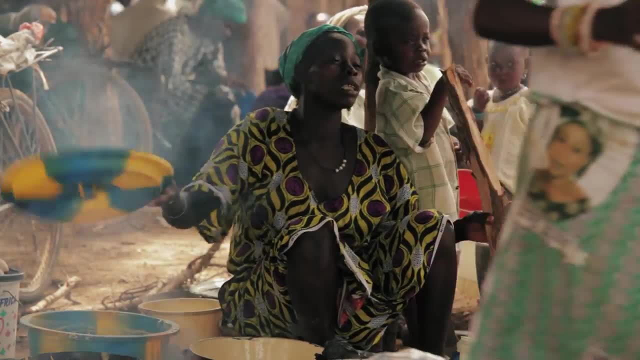 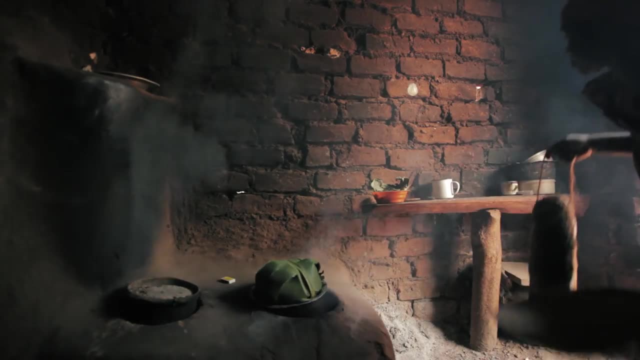 Electrifying the African continent with clean renewable energy would have co-benefits. Reducing the use of wood and other biomass for cooking and heating could reduce pressure on local resources and also improve health through better indoor air quality. But there are challenges.